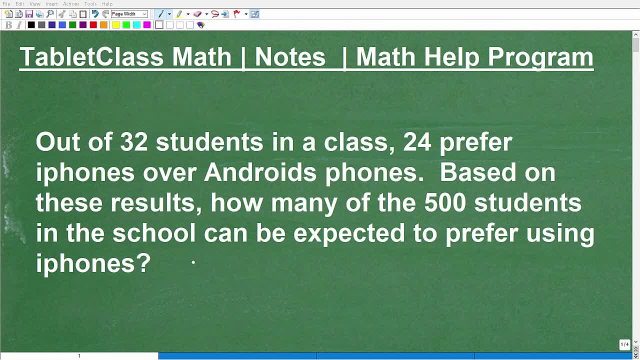 Okay, let's talk about how to solve this particular word problem And this is, I would say, this particular level of math would be appropriate. at least the sixth grade, definitely middle school and absolutely high school students should be able to handle this. But if you're at the sixth grade, middle school level, you certainly will be learning, you know math, these kind of math topics and skills involved to solve this type of problem. 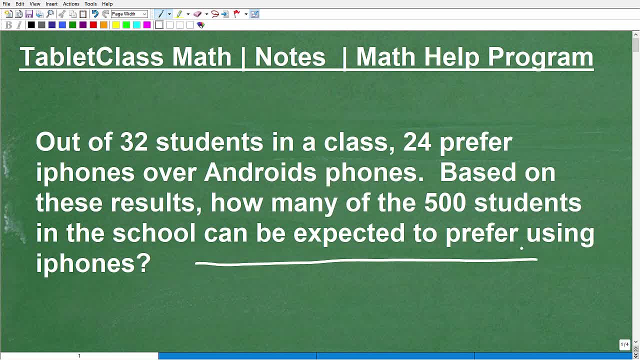 Now I'm going to obviously solve this here in just one second, but I encourage those of you to think about it. maybe pause the video, see if you can solve it. That's always a good way to you know, make the most of my particular videos. But obviously I'm going to solve this And not only that. I'm going to give you kind of a general outline of word problems, how to approach word problems, because you can't have one specific procedure to solve word problems, because word problems are different and require different skills. 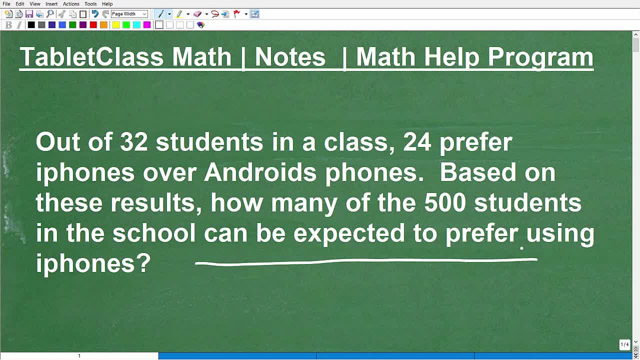 But we can write out a basic outline, a basic general approach that you want to be thinking about. So we're going to get to this particular problem in just one second. But first let me quickly introduce myself. My name is John. I'm the founder of Tablet Class Math. I'm also a middle and high school math teacher And over several years I've constructed what I believe is one of the best online math help programs there is. Of course, I'll let you be the judge of that. If you're interested, you can check out my math help program at following the link in the description of this video. 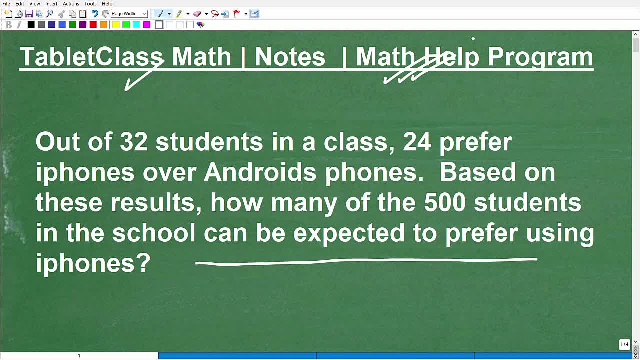 But basically I have 100 plus different math courses. I have all the main courses starting from pre-algebra. So I have pre-algebra algebra one, geometry algebra two. I'm going to be launching pre-calculus here shortly. But I also have many specialty courses in the area of test preparation. So if you're preparing for tests like the GED, SAT, ACT, GRE, GMAT, Accuplacer, CLEP, Alex, teacher certification, nursing, entrance, etc. 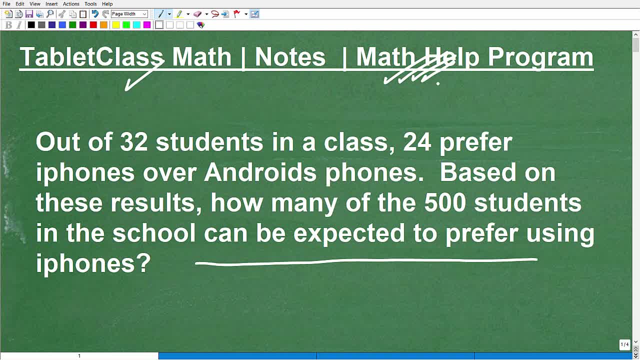 There's a lot of reasons people study math outside of an actual math course. So, anyways, I can definitely help you out. Just go to my site and check out my course catalog. If I don't have the exam you're preparing for, drop me a line and I'll give you my best recommendation. I also work with independent learners, like homeschoolers. I have a great homeschool learning program, So if that's your situation, I can definitely help you out, And then I work with those of you that are needing some assistance in your math class. I could definitely help you out as well. Now I did, or do, teach a middle school math course. 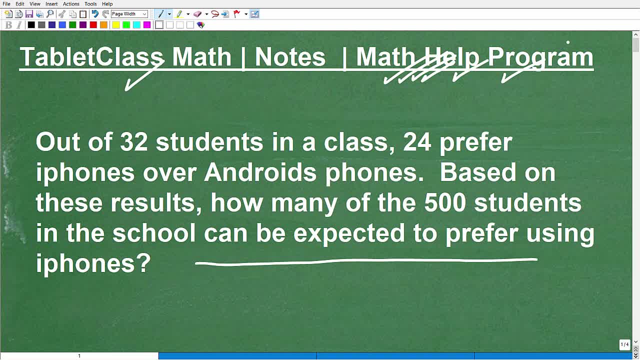 I don't have like a sixth grade math course right now, But my most basic course would be pre-algebra, which I think is still covers a tremendous amount of concepts and topics that you will be learning in a middle school. So that would be my lowest course, if you're interested. But one thing you need to be doing as a math student is be taking great math notes. over decades of teaching mathematics, One thing is apparent to me: those students who take great math notes almost always end up doing great math notes. 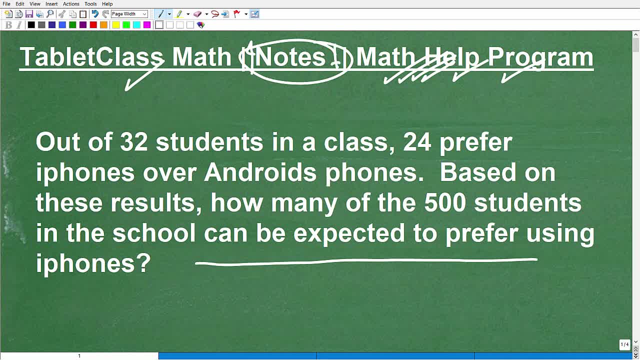 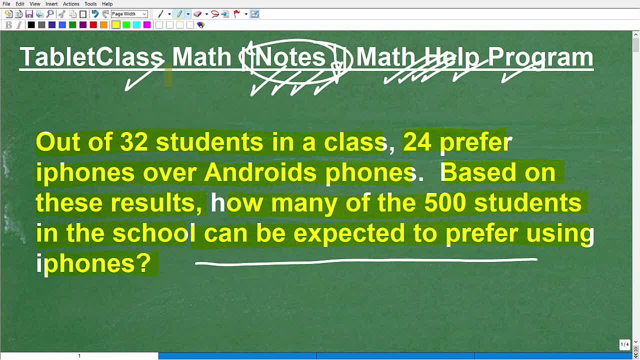 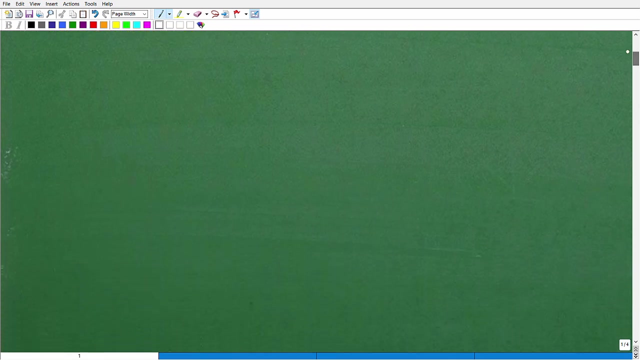 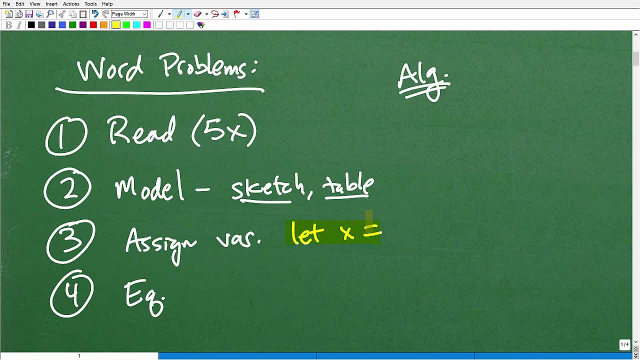 One thing you need to be doing as a math student is be taking great math notes over decades of teaching mathematics really relevant to like algebra word problems. but even at the sixth grade level you are learning basic algebra concepts. so you're going to establish some sort of unknown variable. okay, 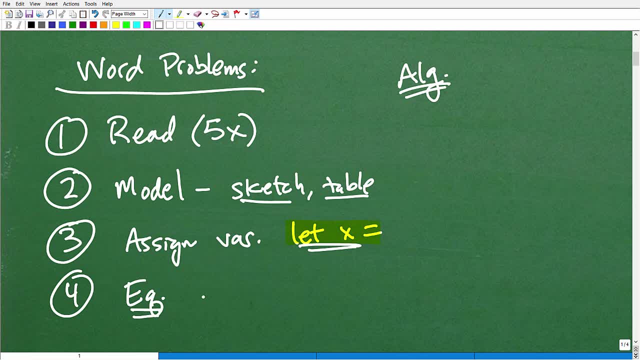 and then you're going to set up some sort of equation to solve for that unknown- let's say it's x, right, then you're going to finish out step five. you're going to solve for what you're looking for- in this case x is some unknown value. and then, lastly, we want to make sure we answer. 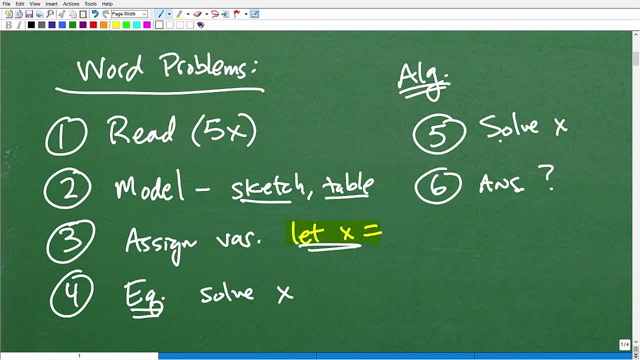 the right question, because sometimes when we answer we solve for this variable, we solve for x. we've got to make sure that in fact it is the answer to the question, and that means we have to read the question again and make sure that what we solve for in fact answers that question. so 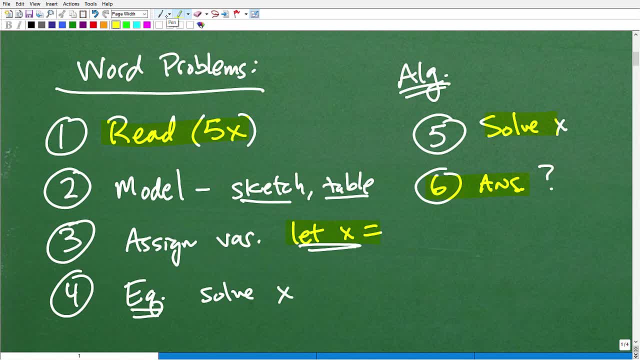 these are kind of general guidelines and you have to adjust them for each problem again. you know this is kind of a sixth grade level, middle school level mathematics word problem. So you won't be using necessarily full on algebra but what we're going to be using here there will be an unknown. 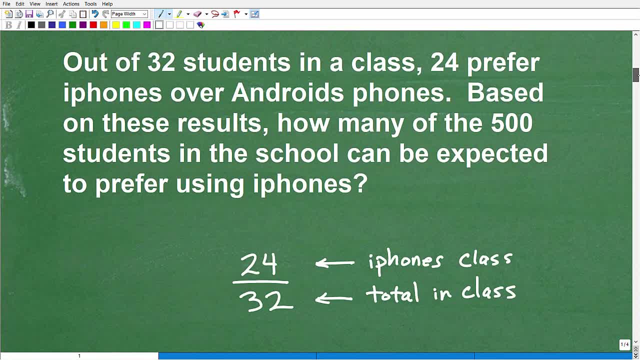 So let's get to the actual problem now. So here it is Right. So out of 32 students in the class, 24 prefer iPhones over Android phones. So let's just stop there and let's see how we can describe this graphically or some sort of way. you know some sort of model. 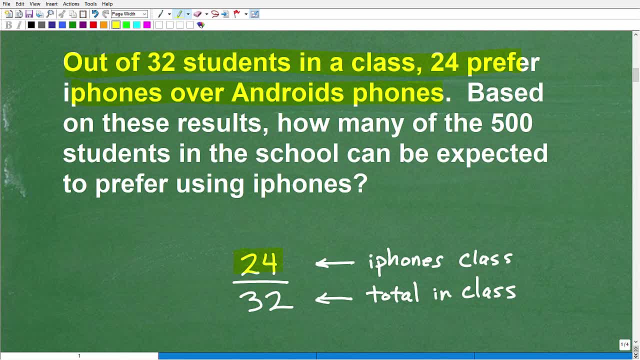 What does this mean? Well, it means 24, OK- out of 32 total in the class. So 24 students out of 32 total students of the class like the iPhones Right, So they prefer the iPhones Right. So this is in the class. 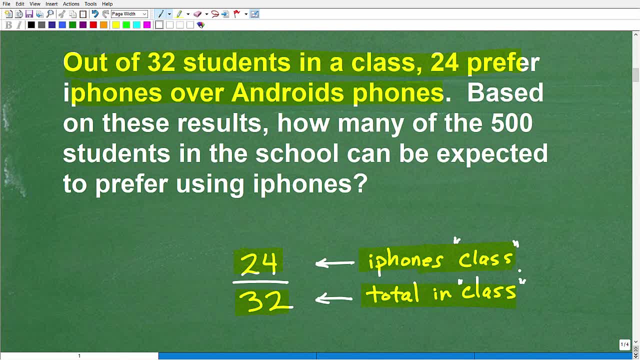 So what we're talking about here- just to kind of tip what's going on is the topic that is involved is ratios, rates and proportions. OK, Ratio, rates and proportions: You kind of like just get a flavor of these type of problems. 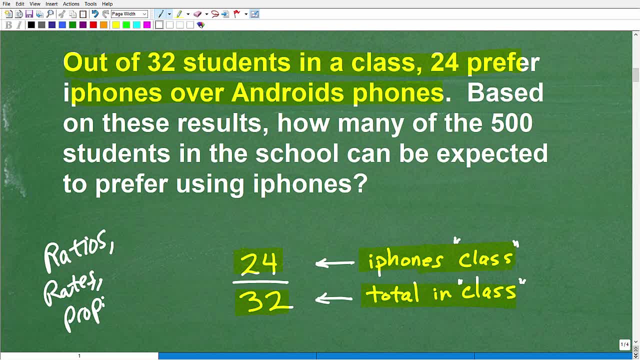 You're like: hmm, this problem seems like it involves ratios, And if we're talking about ratios then we're likely going to be talking about proportions. So this is a very, very- You know- big math concept topic taught at the middle grade level. 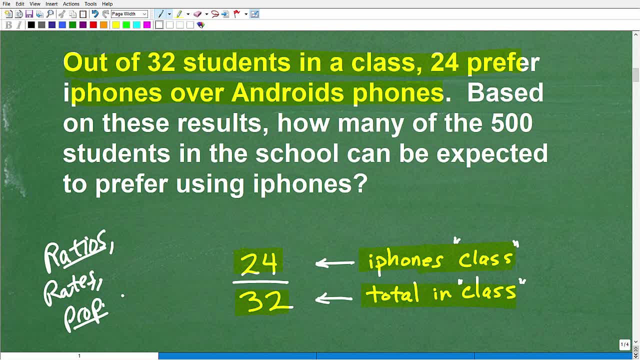 And it's actually just continues on in algebra. It's very, very important, But what we want to do is set up some sort of fraction that expresses the information. OK, so if we have 24 out of 32, let's write it as a fraction: 24 out of 32.. 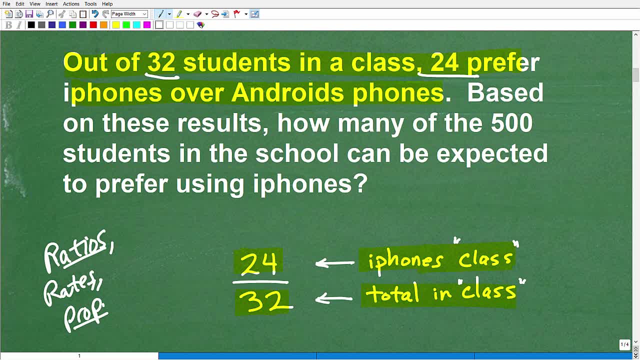 But we have to be very specific on what that means. 24 students prefer the iPhone out of the total of 32.. OK, so we got some sort of you know information down. This would be kind of like our first modeling of the information. 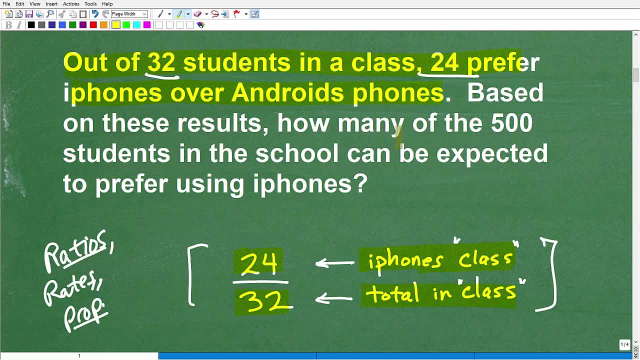 So now we want to move on or read the rest of the problem. So, based on these results, how many of the 500 students in the school? So now we're out of the class and we're talking about the school now. So we have a school that's 500 students large. 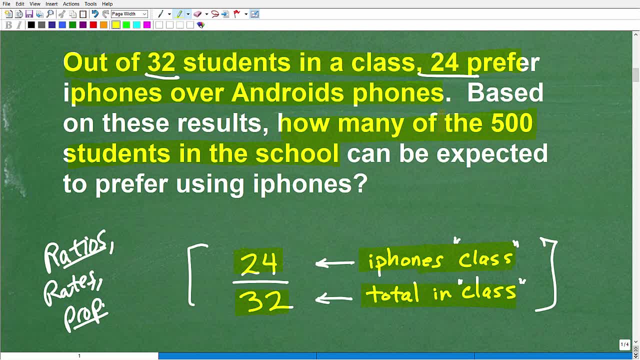 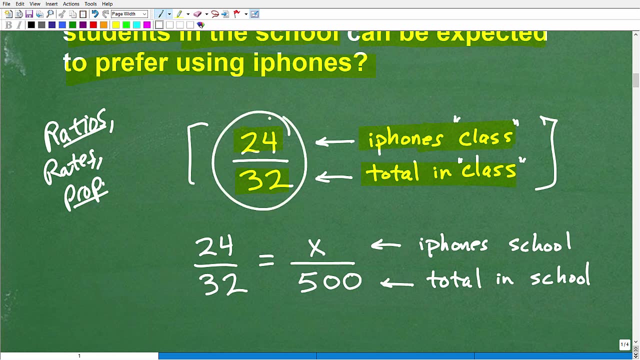 So are the populations: 500 students. So how many of the 500 students In the school can be expected to prefer using the iPhone? All right, So this right here is a ratio. All right Now. this ratio gives us a percentage, if you will, of how many people like iPhones out of the total iPhones in the class, out of the total class. 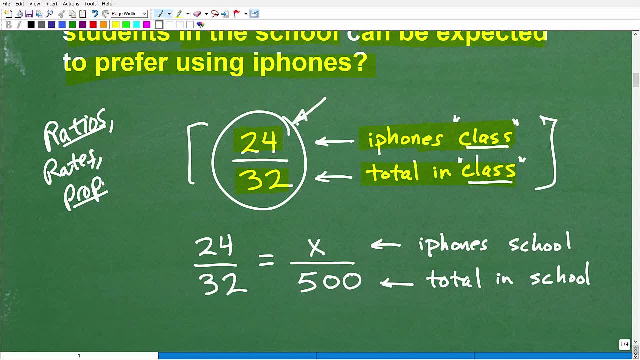 Well, this same sort of ratio, the same sort of percentage, if you will, of people will be the same at the school level, But we need to take this ratio And set up a proportion, OK, so that's what we're going to have to do. 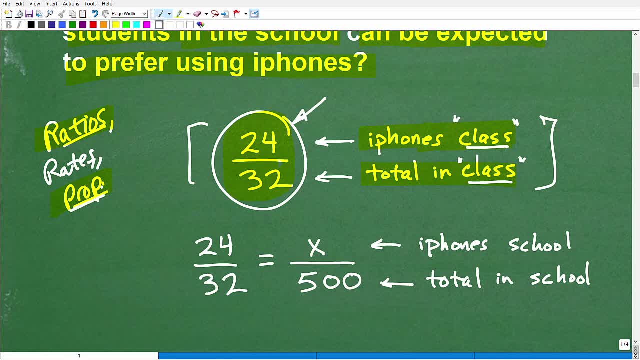 That's kind of the math topic here. So our proportion is two equal fractions or two equal rates or ratios. So we have a ratio here. I want to set it equal to another ratio. So let me show you how we set this up. 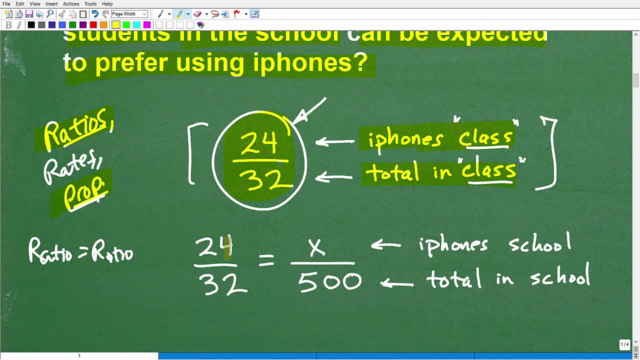 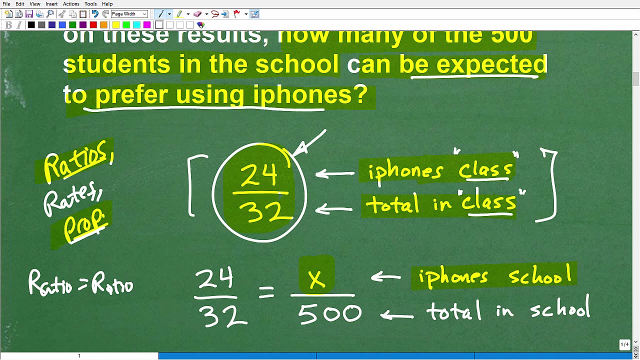 And this would be an example of our equation. OK, now we're going to kind of let X equal the number of people who prefer iPhones in the school, because that is what the question is asking. OK, so how many can be expected to prefer? how many students in the school- not in the class in the school can be expected using the iPhone? 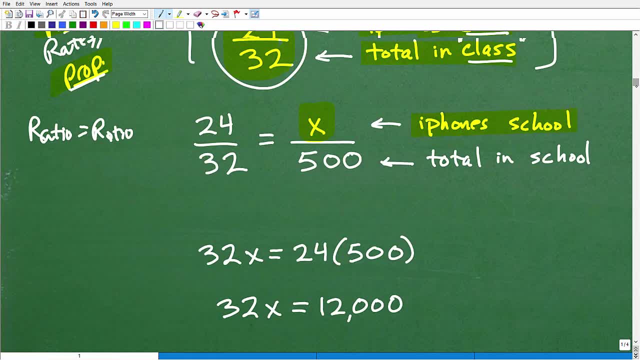 Well, that is our unknown value, or X? OK, so let's write it out here. So let's take a look at how ratios, proportions, work here real quick. So remember, 24 students out of the class of 32 liked the iPhone. 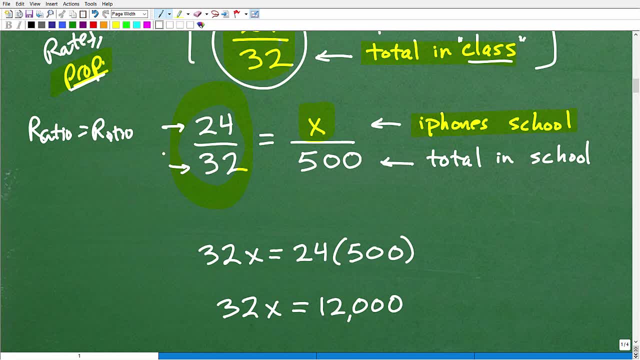 OK. well, this same proportion, or the same, this ratio will be the same ratio in terms of the school. It's going to hold true. So, in other words, it's this fraction is going to be the same as this fraction, But the denominator. this was the total down here in the class. 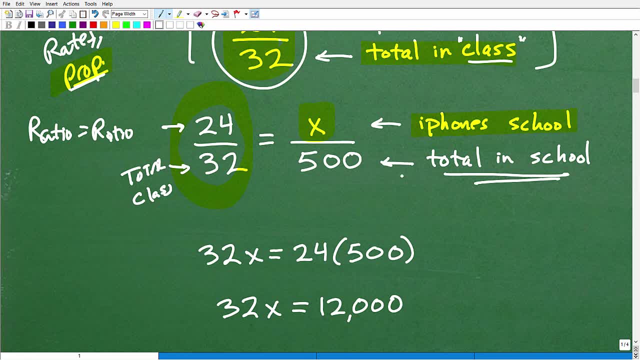 OK, but now we need to involve the total in the school. So, instead of 32 out of a class of 32, think of it as a class of 500.. Right, It's like just a larger denominator. So this is it. 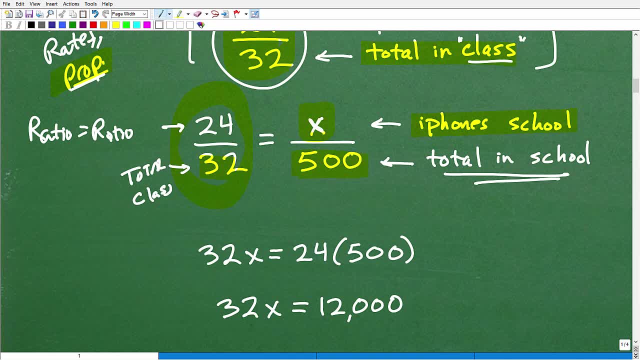 The entire school. But now what we don't know is this: We don't know how many people out of that 500 prefer iPhones, But whatever it is, it's going to be in this proportion. All right, It's going to be the same, equivalent to this fraction or this percentage. 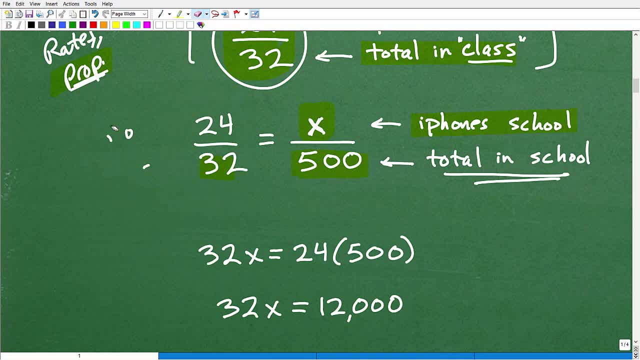 So anyway. so now at this point, OK again. the topic here is ratios and proportions and rates. You need to know how to set one up and what it is And to solve A proportion. So we have 24 out of 32 is the same as some number out of 500. 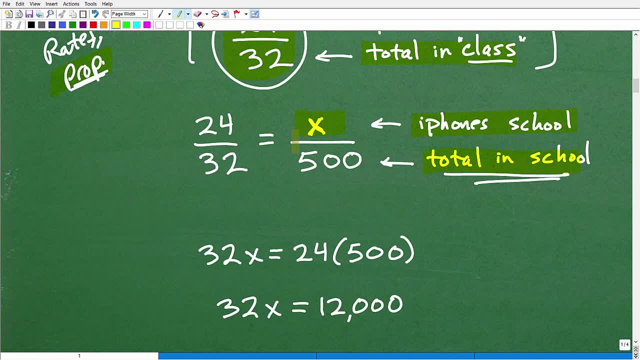 So to wait, the way we solve proportions which are two equal fractions is we just do what they call the cross product. We're going to multiply this way, So that's 32 times X, right there, And then we have 24 times 500.. 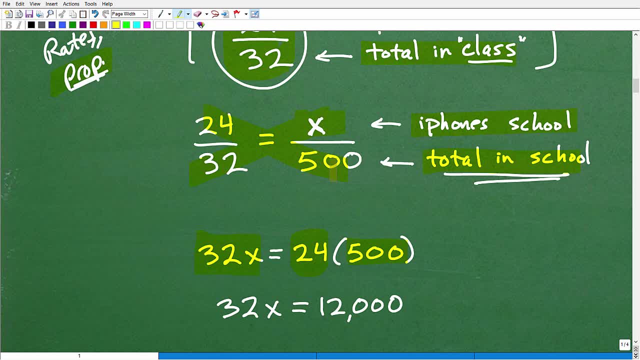 So that's going to be 24 times 500.. So you can do what we call the cross product when we're solving ratios and proportions or proportion prompts. If you need help on this- Ratios, proportions and rates- Check out my videos. 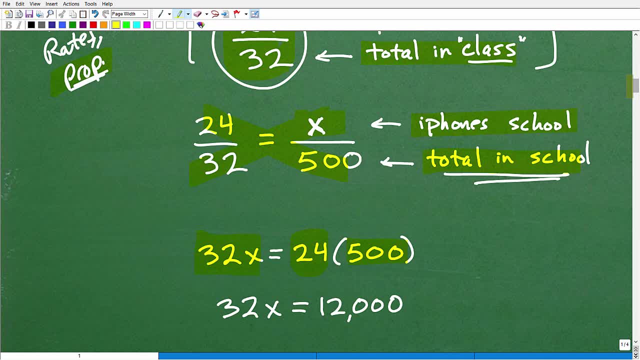 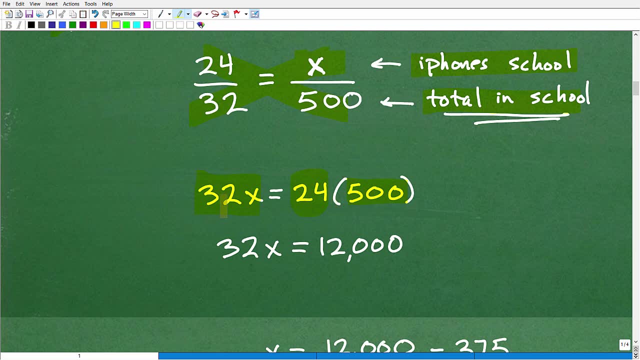 I have a lot of videos in my pre-algebra or algebra playlist or, better yet, just jump into my pre-algebra course. OK, so at this point we need to continue on. We have 32 X 32 times some unknown value. X is equal to 24 times 500, which is 12,000.. 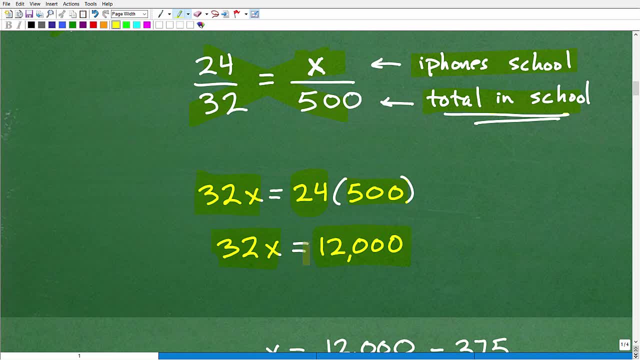 So at the sixth grade level you're learning some basic algebra. Now there are some other ways you can solve this proportion, But this is probably pretty typical, Typical of how to solve it. We don't have to- you know, no full on algebra here to solve this. 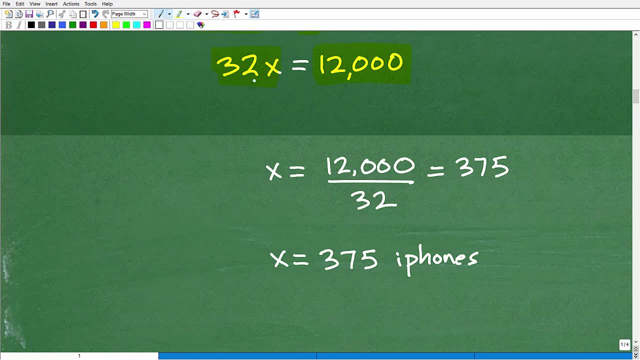 So let's just talk about how do we solve for X. We have: 32 times X is equal to 12,000.. So to solve this equation for X- that's what we want to do- I need to simply divide both sides of the equation by 32.. 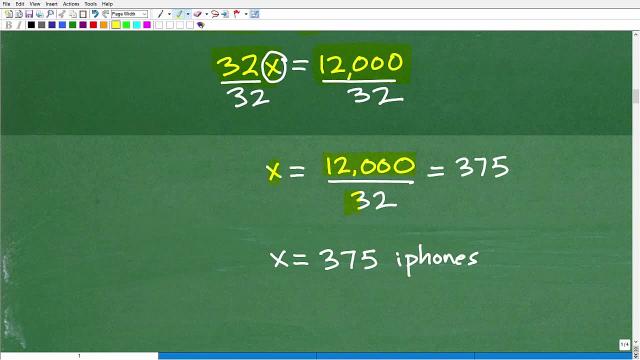 OK, when I do that, I get: X is equal to 12,000 divided by 32, which is 375.. So I solved for X. Now I want to make sure that I understand the answer. I'm answering the question. 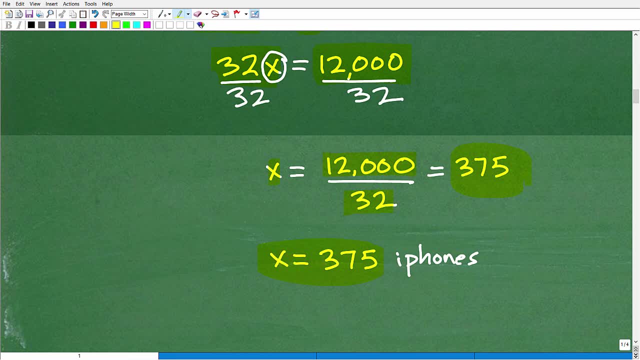 So X was equal to what? Well, that was remember. we had X over 500.. This is how many students prefer the iPhone, OK, out of an entire school population of 500.. So that's our answer. So 375 students actually will just say this. 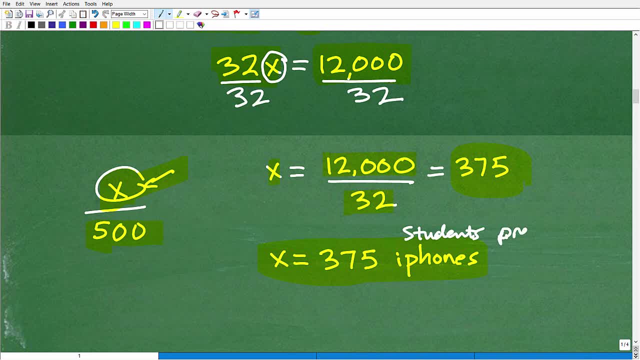 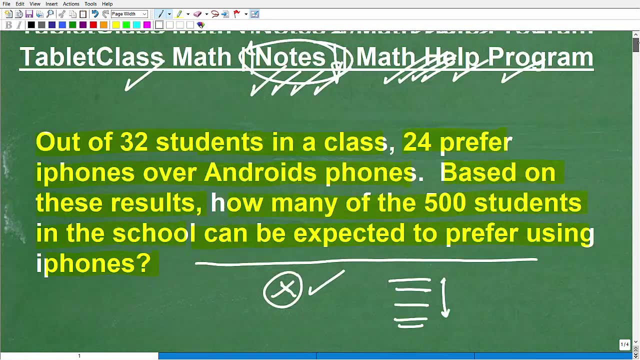 We're specific and correct: Students prefer, prefer the iPhone, and that's it. So if you got this problem right, I would say: wow, that is pretty cool. I would definitely give you a happy face and a plus a 100 percent. 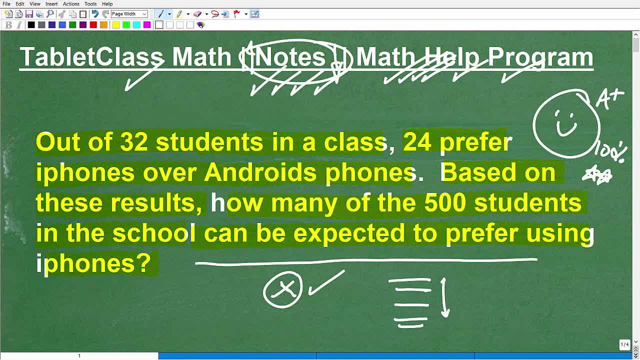 I'd be like: great job, Keep it up, man, Let's throw in a couple of stars. Those are cool too, But that's excellent. OK, that shows me that you have understanding of rates, ratios, proportions, you know. 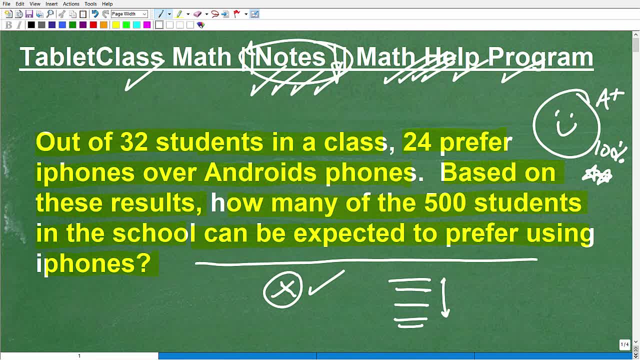 and you can handle work. So this is a, you know, pretty basic level work problem, but pretty, let's say, common at this middle school math level. Now, if you're at a higher level than that and you had a difficulty with this, don't panic.